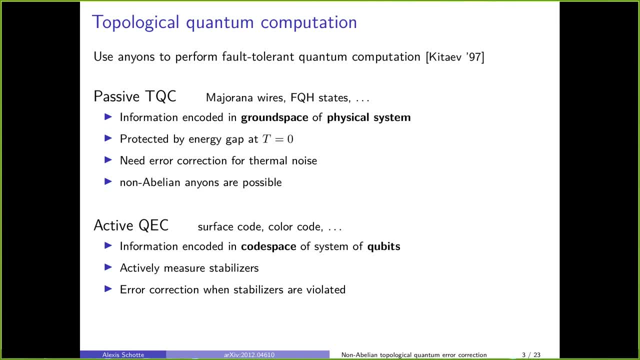 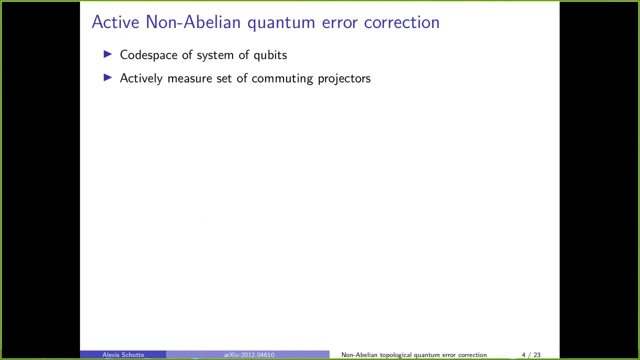 is study active error correction, but with a non-abelian code. So we have a system of qubits and we're looking at the code space defined by a set of committing projectors. These are no longer the product of Pauli operators, But I'll come back on that later. And then, importantly, an important feature is that 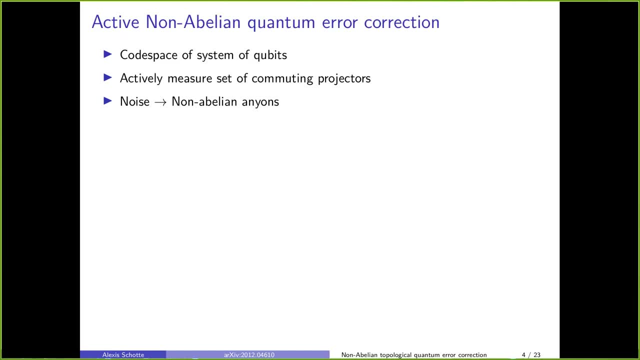 noise will result in some of these projectors being violated and these defects will behave like non-abelian anions. So we have two goals: First, we want to construct such a non-abelian code of qubits and then design all the necessary circuits for measurement and correction. 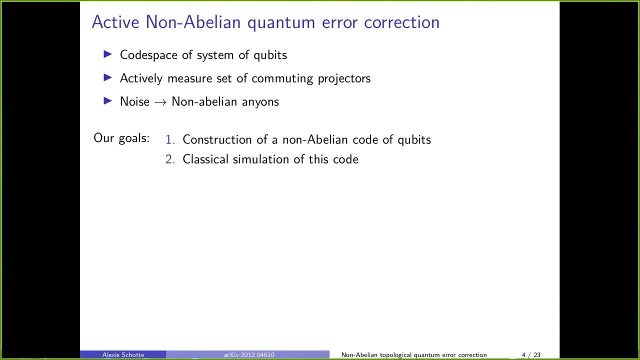 in this code, And then we want to be able to classically simulate this code to find an error threshold. For this we'll be using three things. There is quantum error correction, there is topological quantum field theory, and then there's sensor networks, And it's only by combining these three ingredients that we're 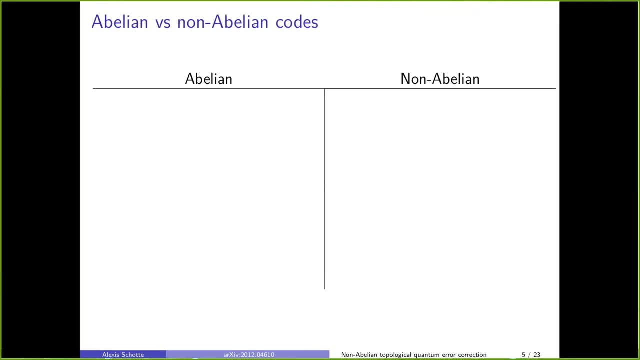 able to solve the problems that we want to solve. So let's let's take a moment to consider the ups and downs of abelian and non-abelian codes. So the upside of abelian codes is that these are very simple in the sense that these are stabilizer codes with low weight, local stabilizers. 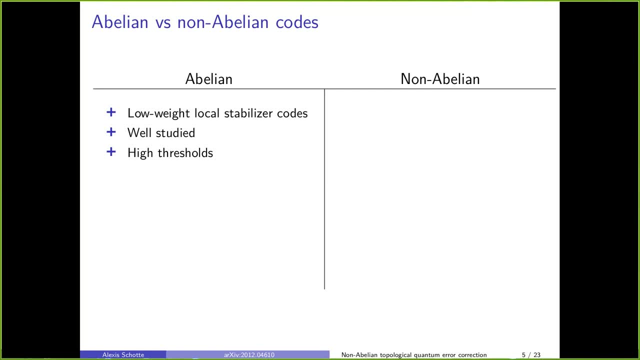 So these have been very well studied, continue to be very well studied and they have very high thresholds. This makes them very attractive candidates for eventually realizing a full, tolerant quantum computer. But they also have a big downside, which is that in two dimensions they cannot perform a full set of a universal set of gates within their code space. 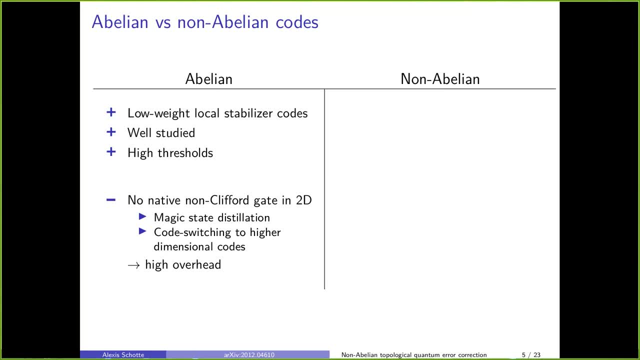 They need to be complemented by some extra scheme to perform a non-clifford gate, either magistrate distillation or code switching to a high dimensional code. It's never free. there's always some overhead when you want to do this. The alternative is non-abelian codes and they have the big advantage that in two dimensions. 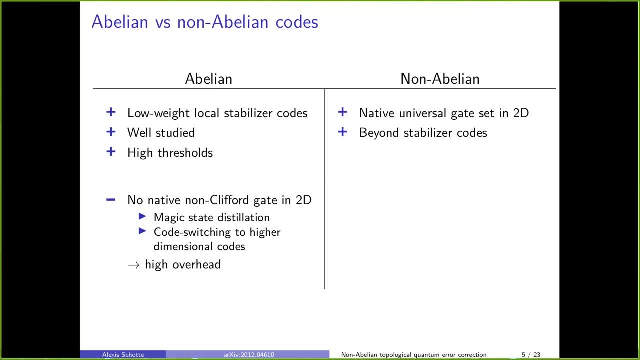 some of them are able to natively perform a universal set of gates. They're also a way to go beyond the paradigm of stabilizer codes. There is no such thing as free lunch, so the price you pay for this is that these codes are. 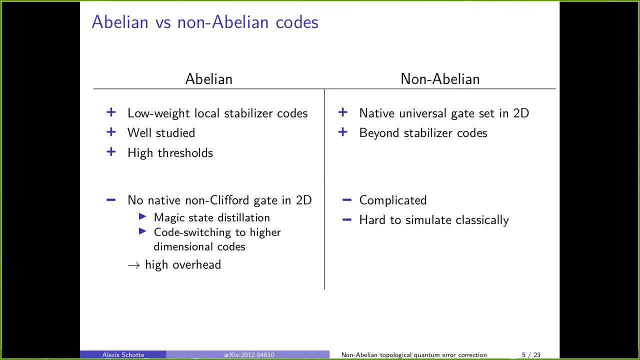 very complicated. As I mentioned before, these are no longer stabilizer codes. instead, they're defined by a set of commuting projectors, and these have a much more complicated structure than the product of Pauli operators. These codes are also very hard to simulate classically. 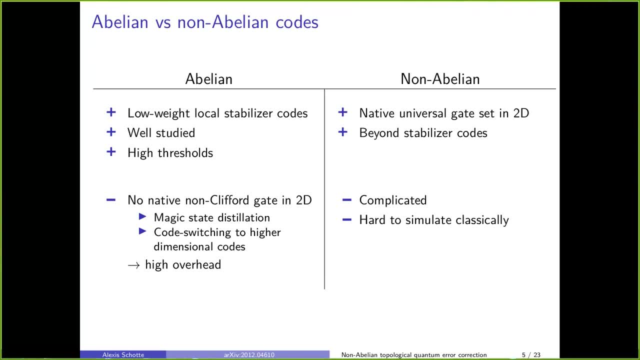 and this is the main reason why there has been very little results on such non-abelian codes. There is very good reasons to study them. it's two dimensional codes with a universal set of gates within their code space. However, they're so complicated to simulate that maybe many people 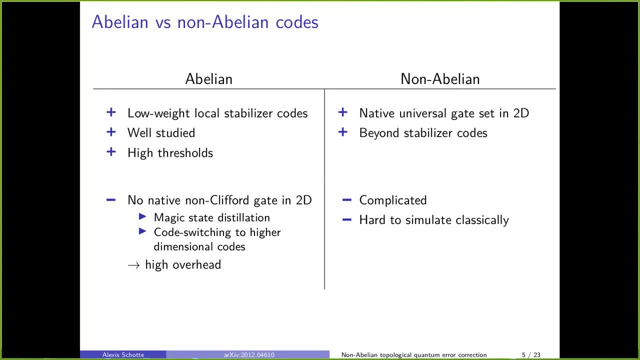 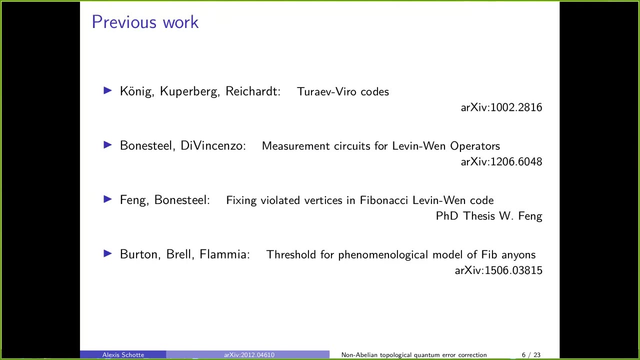 thought that either it would be completely impossible or that, if you could eventually simulate them, that the thresholds you would find would either be non-existent or be very small. We will see that this is actually much better than what people expected. 3. Similarity between non-abelian codes with non-believer codes. 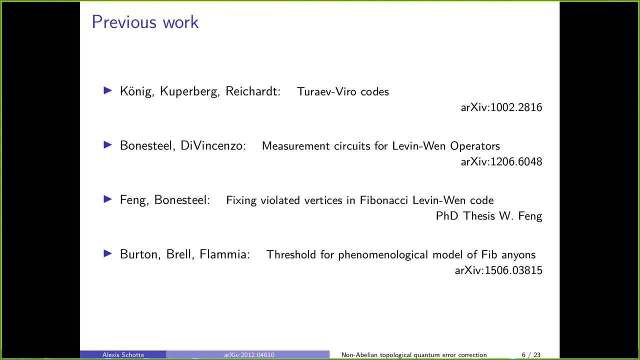 So we're building upon a number of other works, notably the following four. So there is a work by König, Kupferberg and Reichardt where they introduced three high-varial codes. Then there's the work of Bone Steel and DiVincenzo. 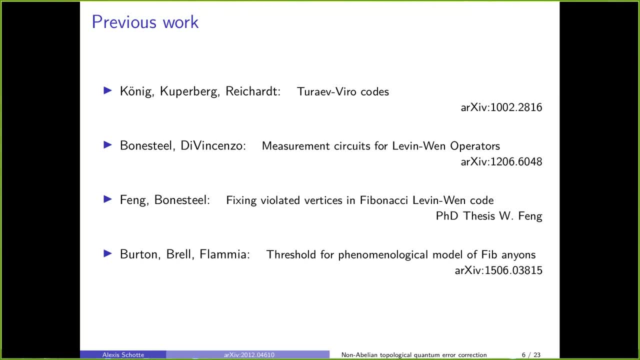 who designed measurement circuits for the Levin-1 operators. There's the PhD thesis of Feng, who introduced some trick to fix violated vertices- I will talk about this later- And then there is the work of Burton, Grell and Flamilla. 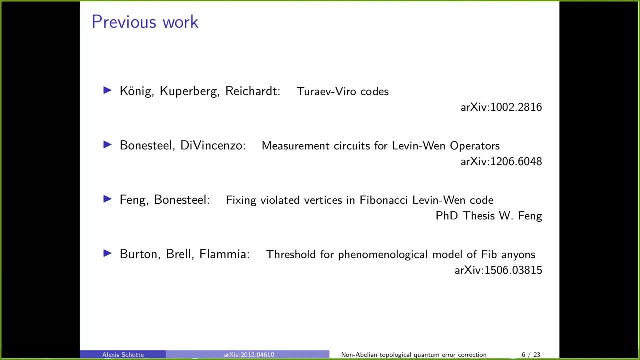 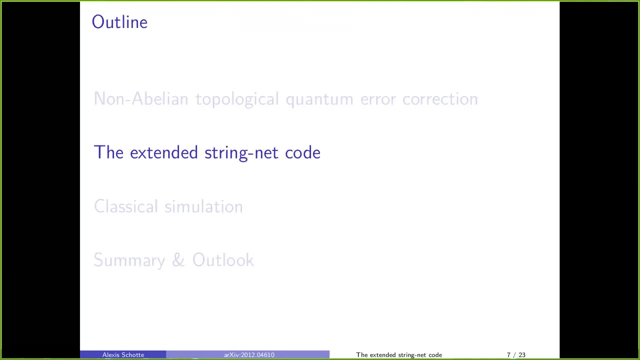 who studied a phenomenological model of Himalayanians and found a threshold for such a code. We use certain of the techniques they use in their simulation to simulate our microscopic model. So let's go on and talk about the code that we used. The code we used is based on the Levin-1 model. 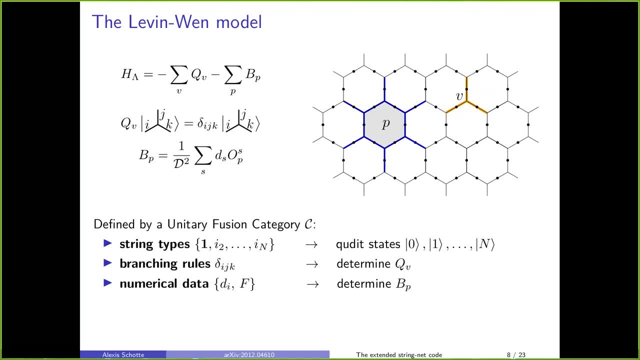 So let's start with the regular Levin-1 model. So it's defined by a set of commuting projectors. There is projectors, There is vertex terms, QVs, And then there is placate terms which in general are 12-body operators. 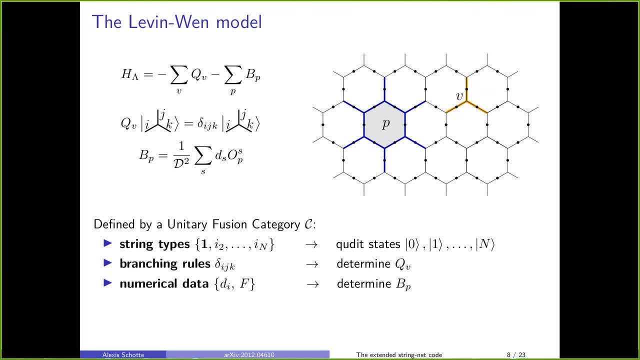 And these are defined using the data of a unitary fusion category. Now this Hamiltonian looks an awful lot like the surface code or the third code, Hamiltonian, And the reason for this is that if you're use the right category for defining this model, you end up with exactly the 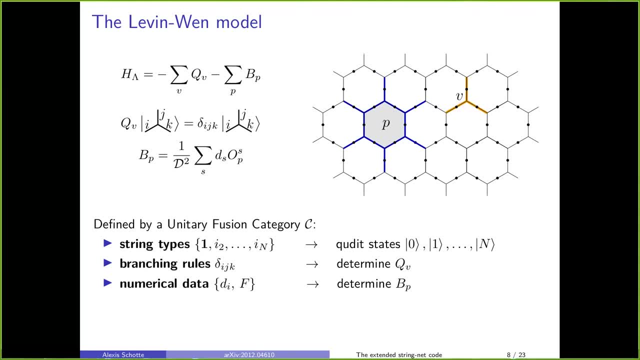 surface code. This is actually a generalization of the surface code on a trivalent lattice. So if you would use the right input category for the surface code, you would see that instead of qubits you have a system of qubits. so you 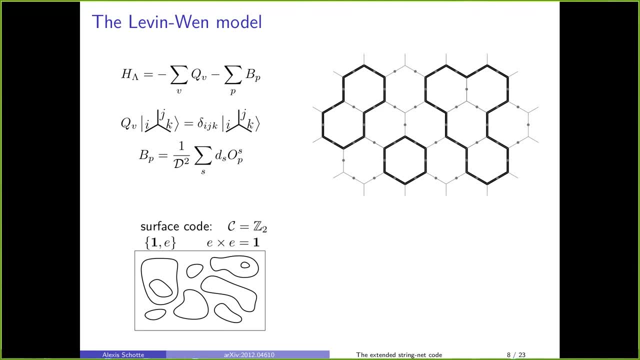 have like two states, occupied and non-occupied, and then your vertex term impose some fusion rule in every vertex, which in this case is that there is no branching or no strings that are allowed to end. So you would get configurations as the one shown here and your ground state is in a superposition. 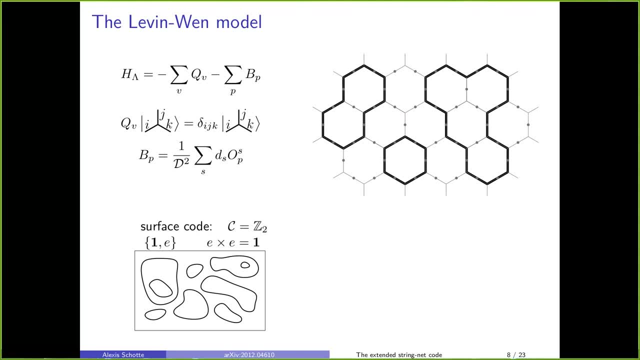 of all types of configurations with loops in all shapes and sizes. We'll be using another category to define our model, the Fibonacci category. This also has only two string types, so it's again a code of qubits, but now there is the. 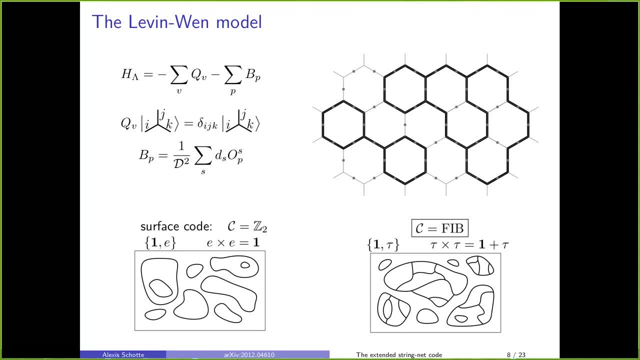 fusion rule that we're going to use to define our model and we're going to use the Fibonacci category. So the Fibonacci category is a function of the superposition of loops, including some branching structure like the one, like the configuration shown here. For further reference, I need to introduce the F. 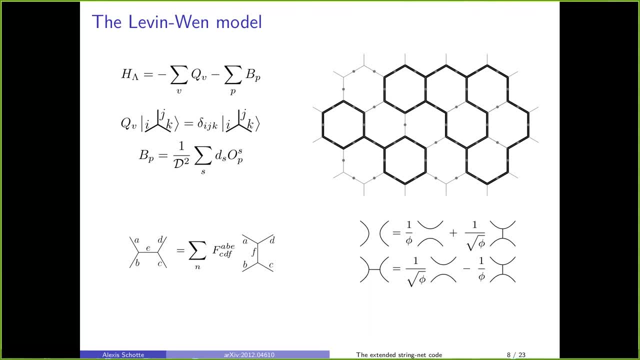 matrix. So the F matrix is something that comes out of this unitary fusion category that you use, and you can think of this as a way of of recoupling your strings, which relates configurations of different loops. So instead of the regular 11-1 model, we'll be using a. 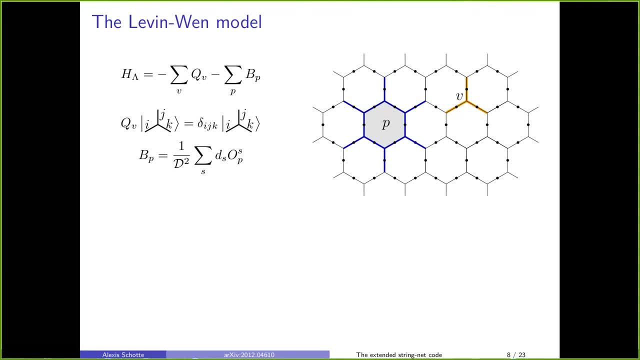 slightly modified one, and this modification is that we add a tail edge inside every placket, So you'll need two extra qubits in every placket. The reason for this will become clear later on, but here are some important properties we will use for this model. The first one is that localized excitations 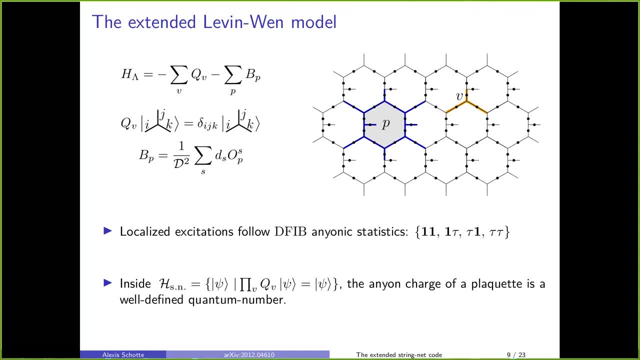 behave like doubled Fibonacci anions. So there's four types of anions. one of them is a trivial one, and then there is three non-trivial anionic excitations. The second property is that inside the subspace, where all your vertex 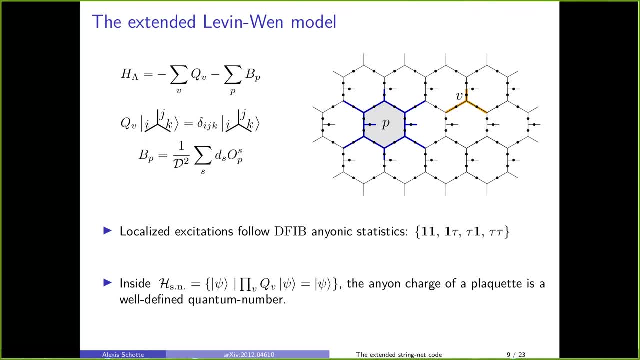 conditions are respected. we call this a stringnet subspace. inside this stringnet subspace the anion charge of a single placket is a well-defined quantum number. So you can write down a projector that projects on the different possible anion charges in one placket The way we 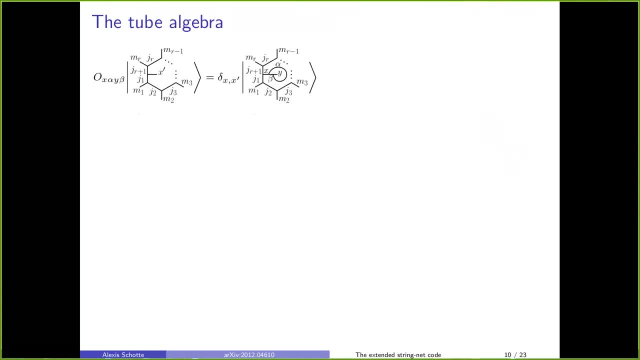 construct these projectors is by using something called tube algebra from topological quantum field theory, and you can think this is an operator algebra. you can think of its generators as gluing this snail-like thing that we call a tube onto this tail edge. So to translate this as an action on these qubits. 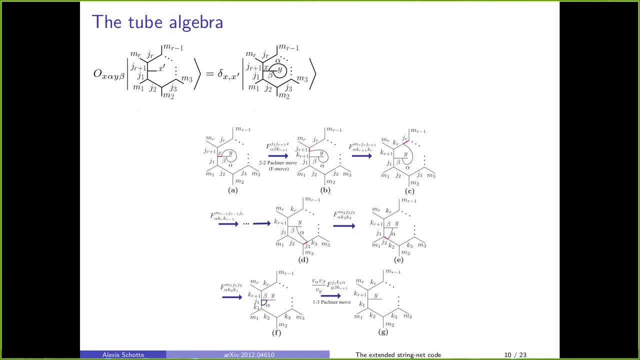 you would use a series of these F-moves to transform the shape back into the normal lattice. So if you do all these steps you would end up with the following operator: And this tube algebra is pretty neat because the very useful thing is that the central 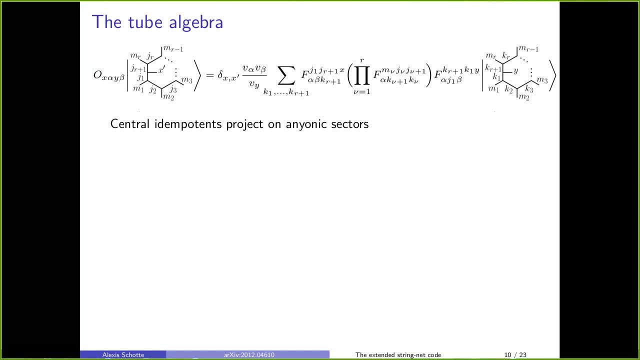 idempotence of this algebra are exactly the projectors onto the different types of anions you can have. So this means that if we combine, if we take the right combination of these operators O, you get projectors on the different anion sectors. So in our case this looks as follows: 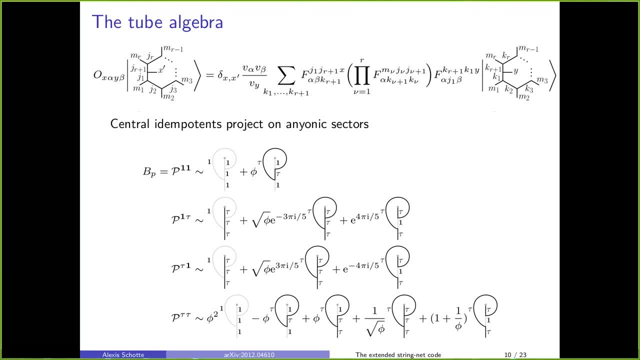 So there is some normalization condition that I left out, But you see, it's just a combination with certain weights of these different types of tubes. Once we have these projectors, this means we need to write down quantum circuits for measuring these things, And this looks as follows: 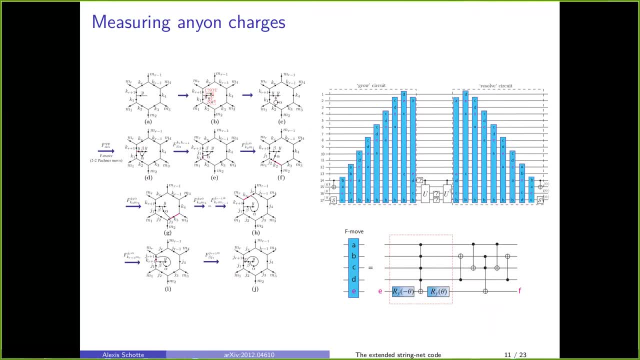 So these blue blocks on the right, they represent a single F-move. So this is the gate that performs this F-move that I mentioned a few slides ago. So what you would do is you would use an ancilla that you would entangle and you would use. 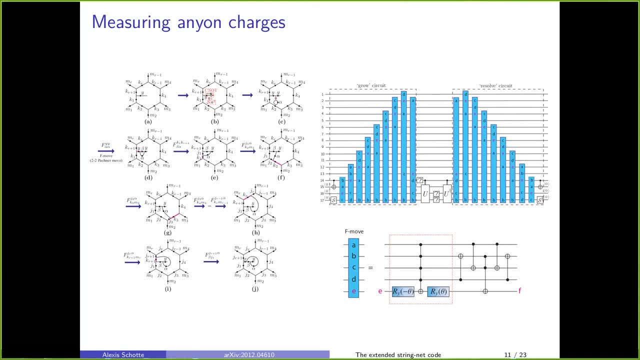 this to grow a bubble, which you would then stretch out by a sequence of F-moves until you get this tube shape. This would then be measured in the appropriate basis And then you would do the inverse of all these, of this first half. So you do all these F-moves in reverse. 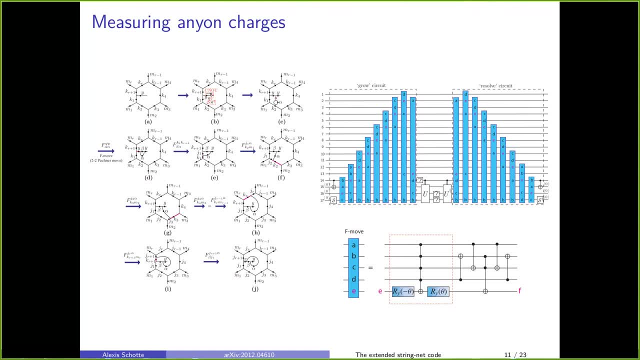 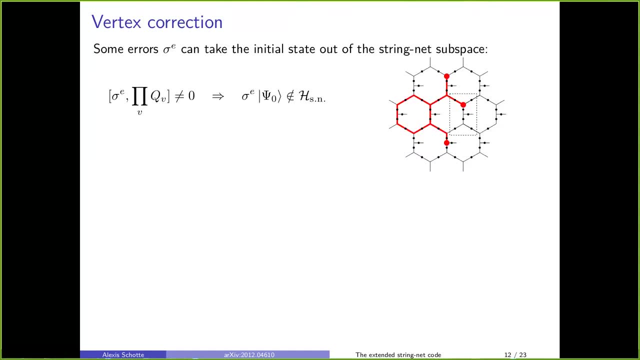 to get back to your original lattice. So this is a pretty big circuit, but it can be cut in half using some tricks, But this is the cleaner way of doing this. So the things I mentioned, so let's go back. These circuits I mentioned are for measuring. 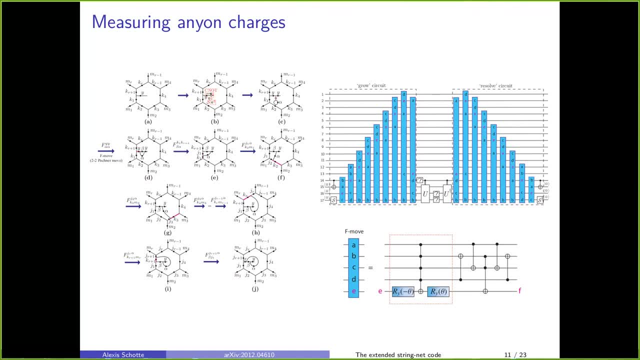 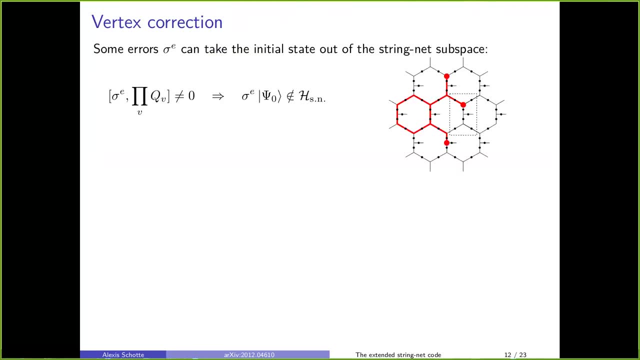 the anion label or a plaquette, But this is only well defined within the subspace where no vertices are violated. So, of course, when your code is subjected to noise, it's very well possible that some error happens and will take your state out of the subspace, And this seems like a problem. 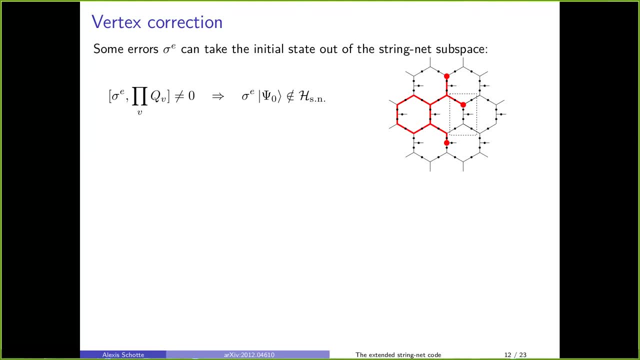 but it can be solved, since if you measure all your vertices and all these tail qubits as well, then you can condition some unitary data. So it's easy to train. but I think this is something that you would do in your class, So this seems like a problem, but it can be solved, since if you measure all your vertices and all these tail qubits as well, then you can condition some unitary data. So this is the cleaner way of doing this. 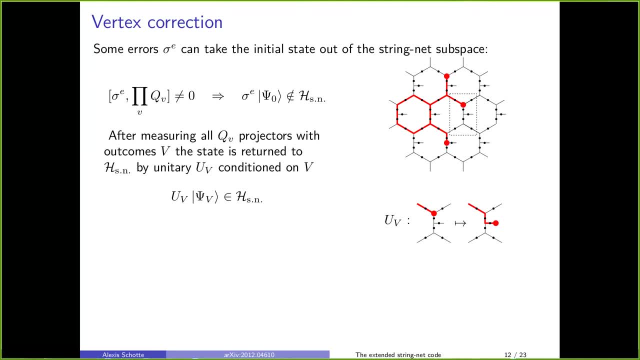 operators all these measurement outcomes to get your state back into the stringless subspace. So what we do is we measure everything and then, depending on the outcome, we apply the right circuits to get back to this stringless subspace by fixing the violated third issues. So here's: 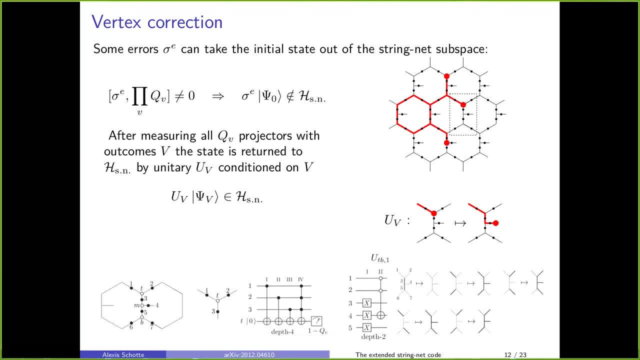 an example of such a circuit and the left is just a labeling of the difference of the different qubits and the middle part here is just the measurement circuits for a vertex term. This was designed by Bonsi and DiVincenzo and here on the right is an example of this vertex fixing. 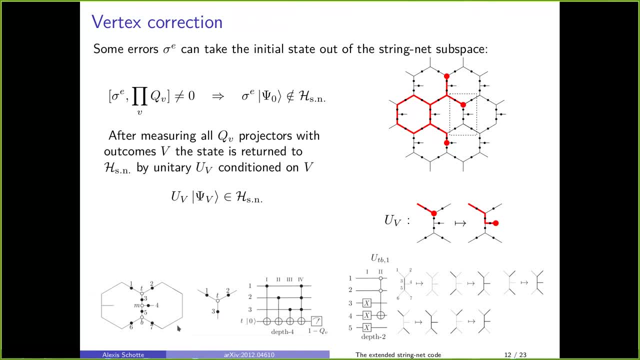 So if on the picture on the left you would find that the top and the bottom vertices are violated and you would find that your string qubit or your tail edge- sorry that your tail edge is in the zero state- then this would be the circuit to fix it. As you see, this is a pretty 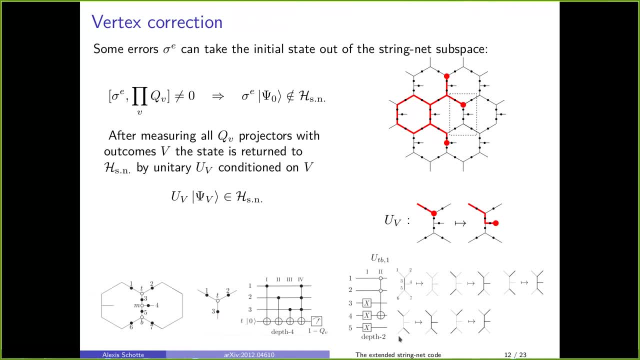 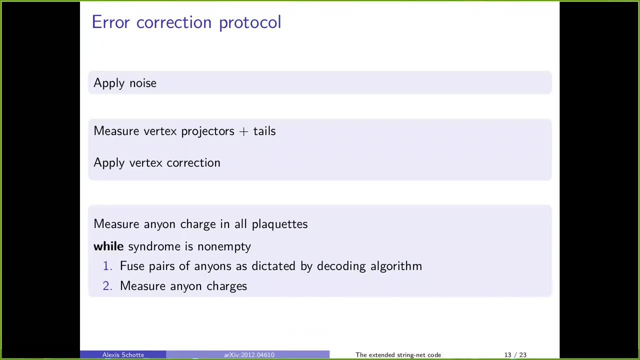 simple circuit. it's just flip three, four and five. except if one and two are both in the zero state, then only flip three and five. So all all different possible circuits that you can need are all pretty small. the biggest one only has depth four. So in general there are correction protocol splits in two parts. well, 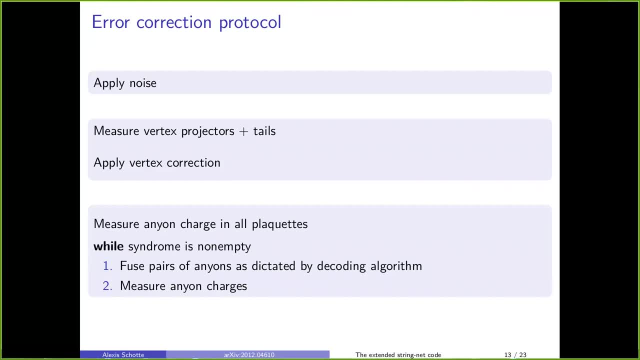 once your system has been subjected to some noise. you would then first measure all your vertices and all these tail qubits, then, depending on the outcome, you would apply the right vertex correction and then you're back in the stringless subspace. So then we can go on with the second part. 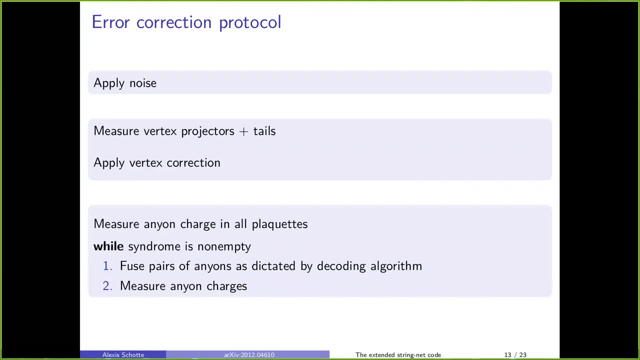 which starts by measuring the alien charge in all your products, which starts by measuring the alien charge in all your products, and then, if you find any non-trivial onions, you would give this information to your decoder and your decoder will tell you which pairs of onions to fuse along which parts. 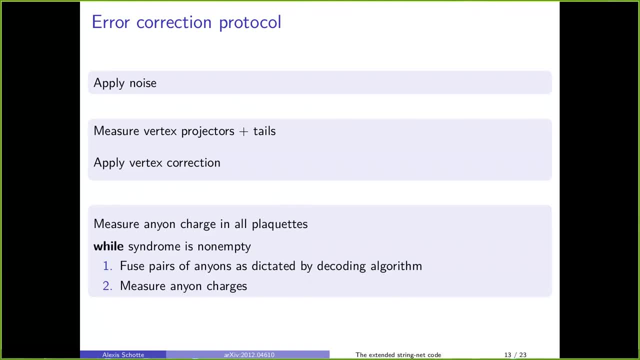 You then do these fusions and then you measure the fusion outcome. since this is a non-abelian model, the fusion outcomes are not determined beforehand, so you need to measure whatever comes out of these fusions. You then feed this new information to your decoder. it will give. 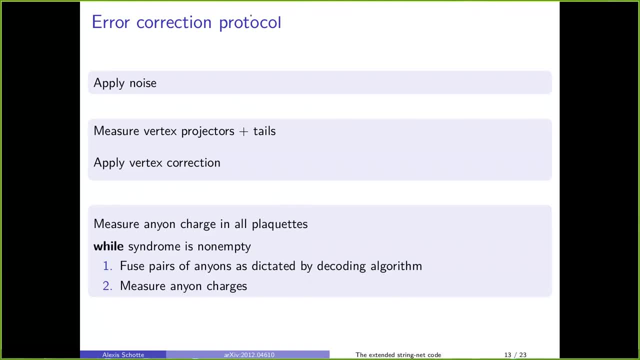 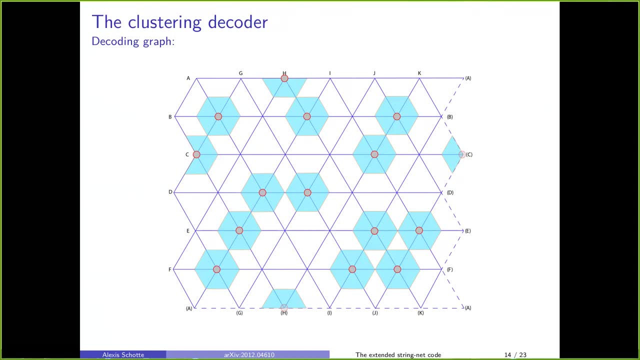 you new pairs of onions to fuse, and so on. So here's an example of such a decoder, and so a decoder we call the clustering decoder. this is not something we came up with. it's an existing model, and so this is a decoding graph. so every vertex here represents one plaquette. 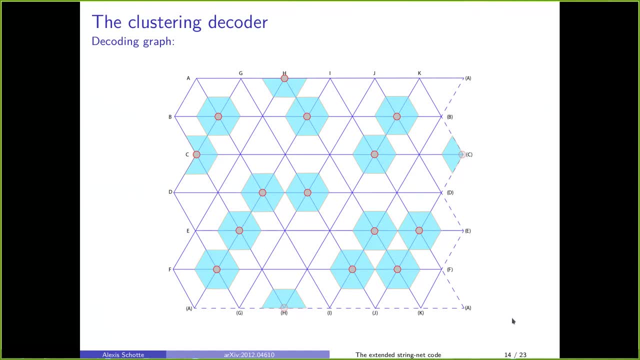 in your actual model. so this packet may or may not contain onions, and the ones who do have been indicated by these, these gray dots. so you would grow a cluster around each of these affected plaquettes and then you would merge all overlapping clusters, fuse all onions inside each of these clusters and measure the. you would then measure the fusion. 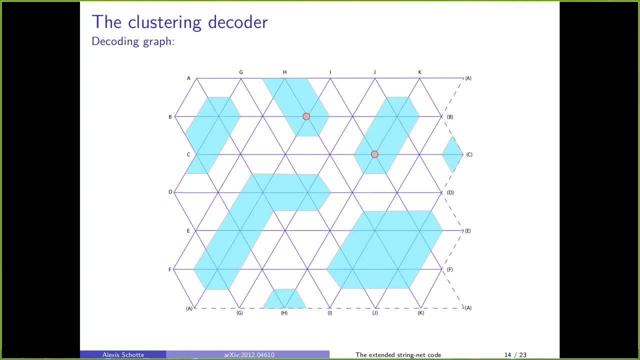 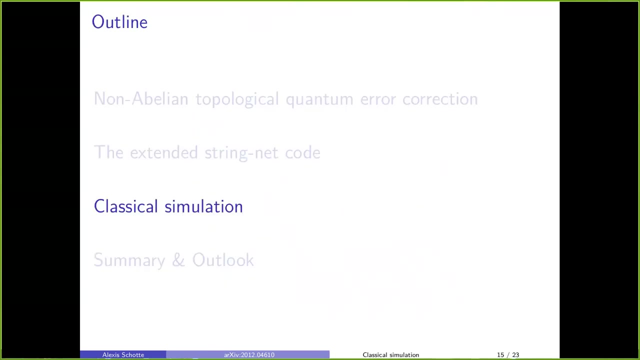 outcome. so here there's only two of them that did not fuse to the vacuum and they would grow. all the clusters merge the overlapping clusters, and then you are at the beginning. so you fuse all onions within each cluster, and so on. So if you want to classically simulate this code, 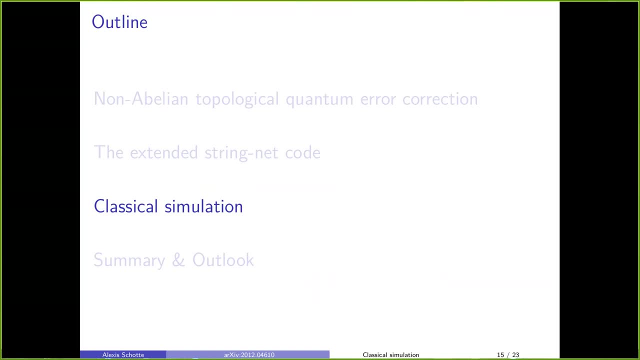 so this is the. this is the hardest part of this thing. you cannot just keep track of the state of all your qubits, since, of course, this would be much too complicated. instead, we need some way to translate noise on the level of individual qubits to processes involving onions. so, instead of keeping track of 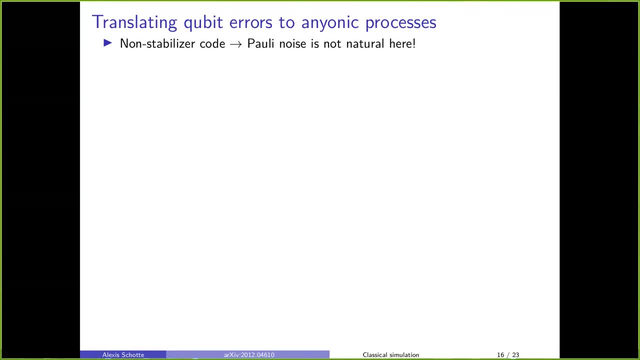 the full state of all your qubits. you then keep track of the fusion state of the onions that get created by your noise. to do this we use the fact that fusion states of onions in your different plaquettes. so the red lines represent the fusion tree of onions in different plaquettes and these fusion states have a one-to-one. 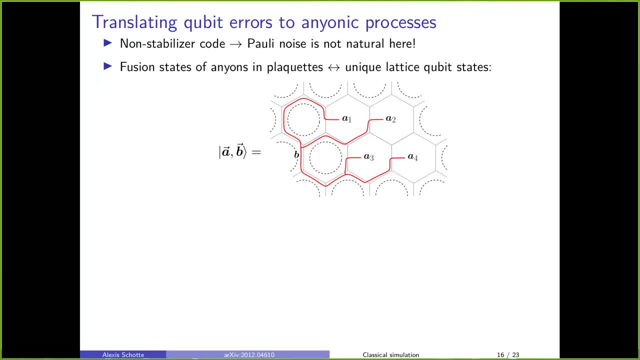 correspondence with states of your qubits. these are then very complicated superpositions of qubits, but there is an exact correspondence to a fusion state with onions and a superposition of qubit states. furthermore, if you take a fusion tree which includes all your plaquettes, 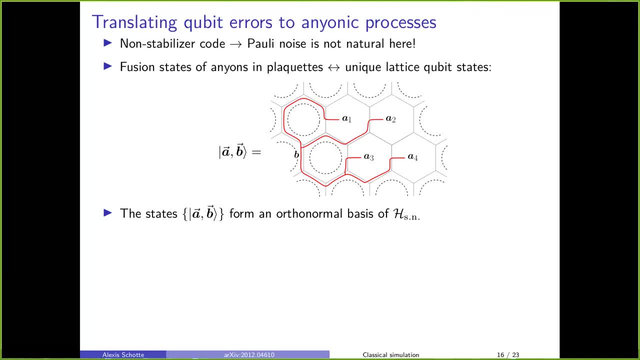 all labelings of this fusion tree corresponds to a set of states which is exactly an orthonormal basis of this stringnet subspace. so this means that this translation between noise on the level of qubits and processes with onions is just a basis transformation. so what we need to do is we 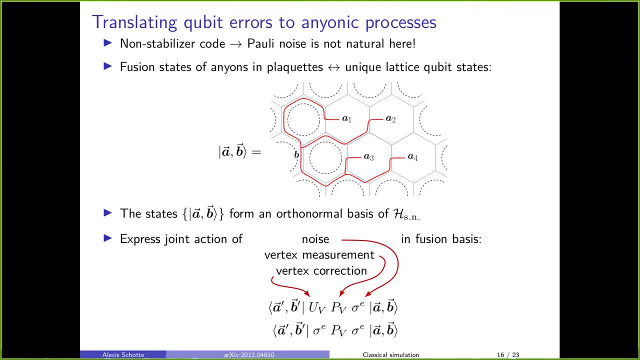 need to express the action of noise, vertex measurement and vertex correction in this anionic fusion basis. so we need the following matrix elements, once shown here below for those wondering, the bottom one is necessary in your simulation since you need a way of sampling measurement outcomes for vertex measurements, so you need this probability distribution. 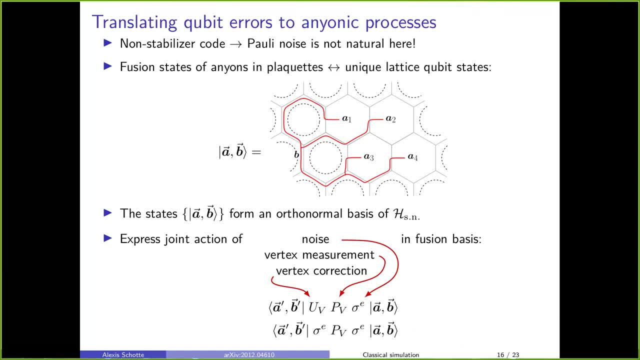 so after computing. well, so the question then, first, is how do we compute these things, since these, these fusion states, are extremely complicated if you consider them in your computational basis of your qubits. so this is how we compute these distribution states and, at the topic of a moment, 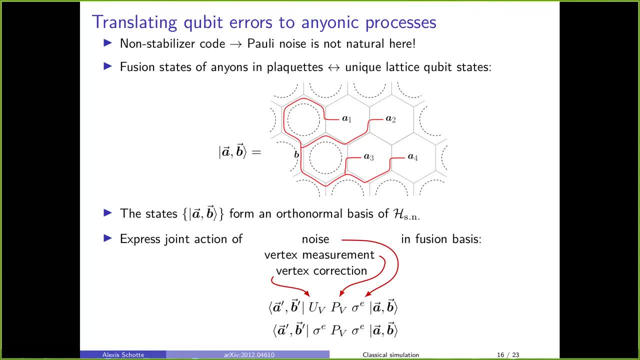 here we go to a backstage where we will understand the making of these distribution states as features, app indents, of the abilities of those properties to helps. to apply the cheapون to the shaping function is a very non-trivial task, so we'll be using two things to do this. First, these matrix elements. 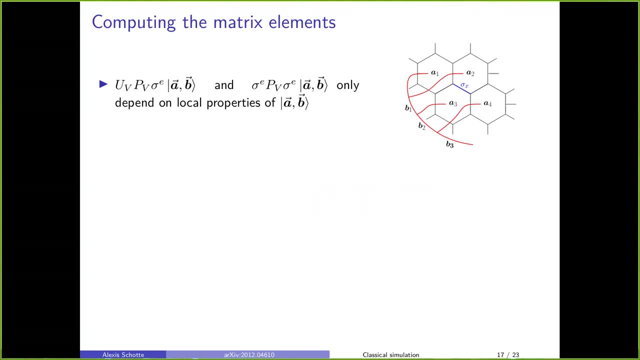 should only depend on local properties of your state. They should not depend on the onion charge of some placket far away. So for example, here on the right is the case of a sigma Pauli x error. It should only depend on the onion charge of the plackets right around it. and then 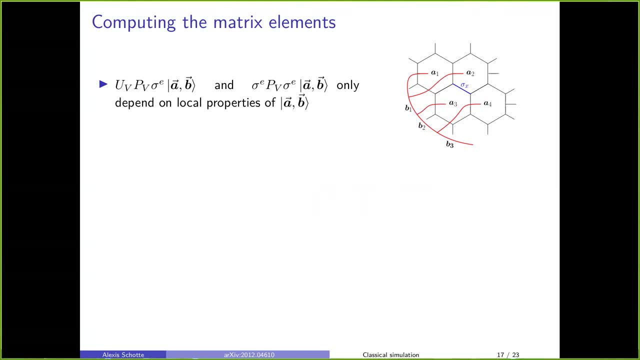 the way in which these can fuse in their total charge. It should not depend on anything else. The second thing we use is that these complicated states can be expressed as a tensor network state. And these tensor network states, they have the same structure as this fusion tree on the virtual level. So by using these two points and then throwing 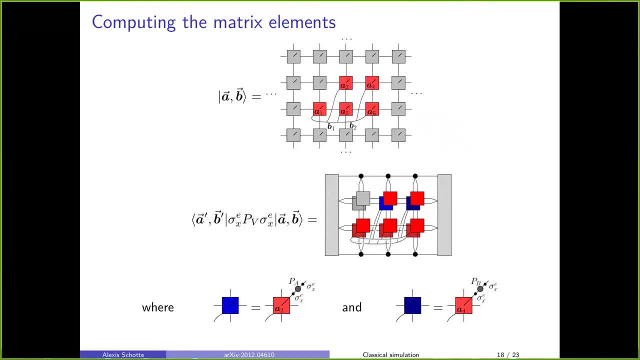 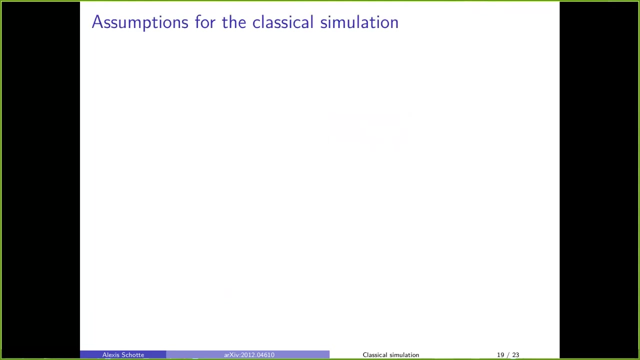 a whole lot of tensor network machinery. at this, you find that these matrix elements can be calculated as the contraction of a finite tensor network, And so, with enough care and patience, you can calculate more or less all 8.7 million of the non-trivial ones, And then you can use this to classically simulate the effect of noise. 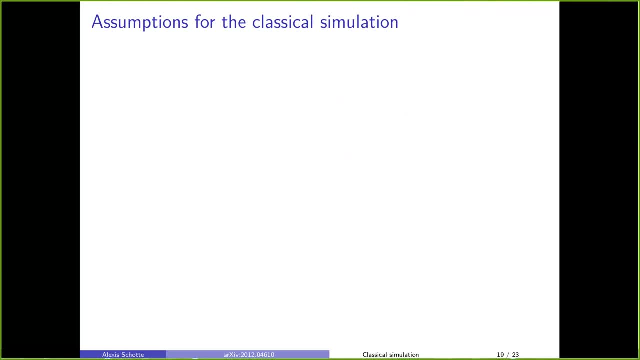 on your model. So here's the assumptions of the simulations we did. First, noise is represented by random Pauli errors on individual qubits. The errors on single qubits follow some Poisson process with a fixed rate which we call p. So the total number of errors which we note here as t will follow some Poisson distribution. 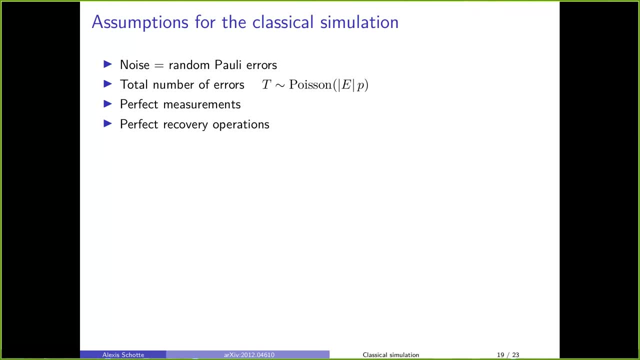 with the mean given by the product of the number of qubits in your system times, the rate of the errors on each of them. We assume that all measurements are perfect and instantaneous And we assume that the recovery operations are also perfect. So our simulation would work by. first you pick the number of time steps that you're going to. 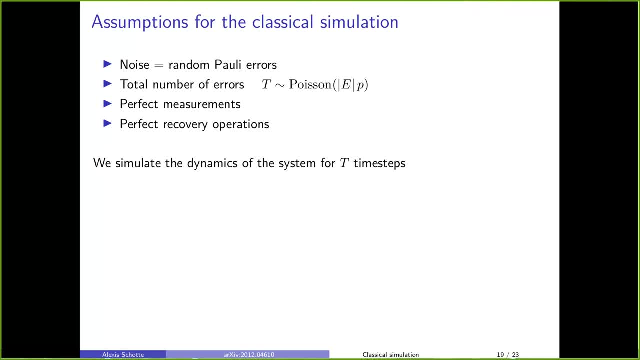 simulate. So t speaks from this Poisson distribution and it's the number of errors that will happen on different qubits. Then, each of each time, step in your simulation consists of the following steps. First, you select some random edge, so some random qubits. 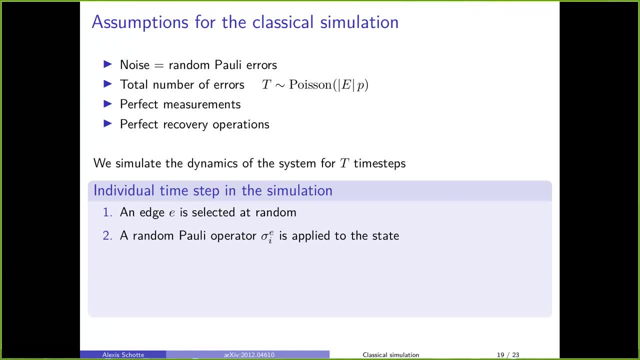 You select some random Pauli and you apply it to this error, to this qubit. Then all vertices are treated with a second time step correction, then all vertex terms and all tail qubits are measured. Then, depending on the outcome, the right unitary to correct the violated vertices is applied And then finally, 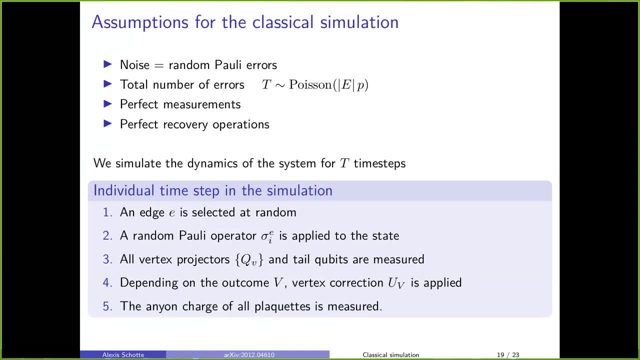 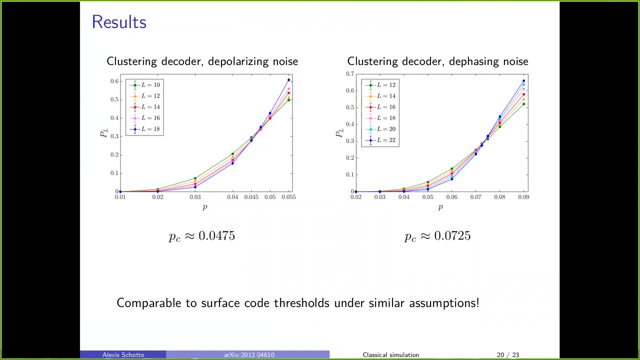 the onion charge of all your packets gets measured. So with these assumptions and using this cluster decoder which I mentioned earlier, we get the following results. So these plots here represents on the x-axis. you see, this is the error rate of an individual qubit. 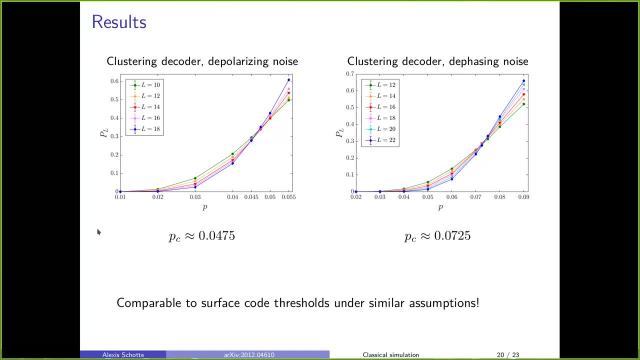 And here we show the logical failure rates on the y-axis. Different curves correspond to different system sizes. By the way, I forgot to mention, this is our code is put on a torus, So you get. it's like the generalization of the toric code, essentially. 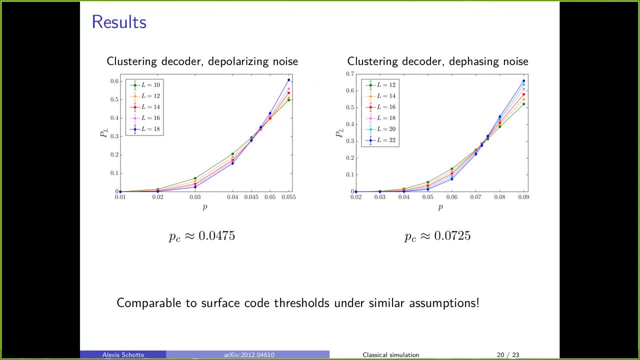 And so L here is the length of the shortest cycle in your torus. And then what we see here is very clear threshold behavior. And not only is there a threshold, it's actually really high. So people expected the thresholds to be non-existent or very low, And what we see is 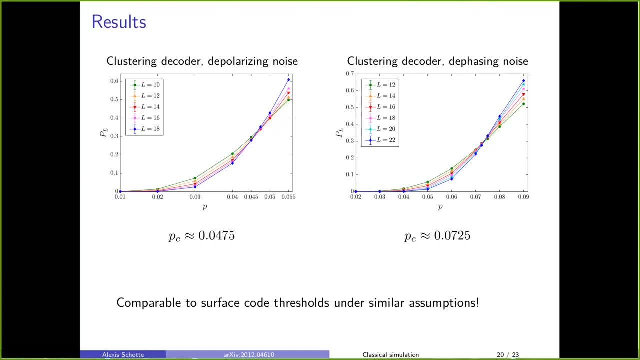 for depolarizing noise, we find 0.0475.. So this is comparable to the surface code with similar assumptions. So this is not only surprising, it's actually very good news, especially when you consider the fact that this is done with just a Monte Carlo simulation. 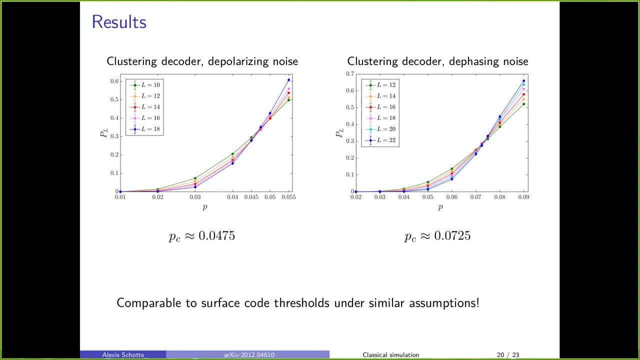 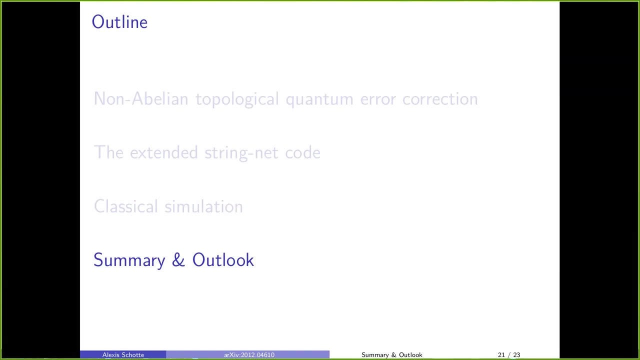 with some decoder. This is not some analytical bound on the optimal thresholds. There might be other decoders which do better than this. So let me conclude with a summary and then some ideas for where to go from here. So we studied active non-abelian quantum error correction. So it's a system of qubits. 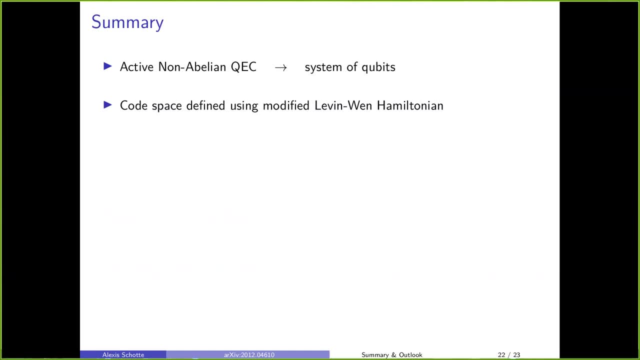 A code space defined as the ground state of a slightly modified Levene 1 model. We use three things: We combine quantum error correction, topological quantum field theory and tensor networks, And only combining all of these could we find a threshold. And this is actually the first threshold for a code in two dimensions. 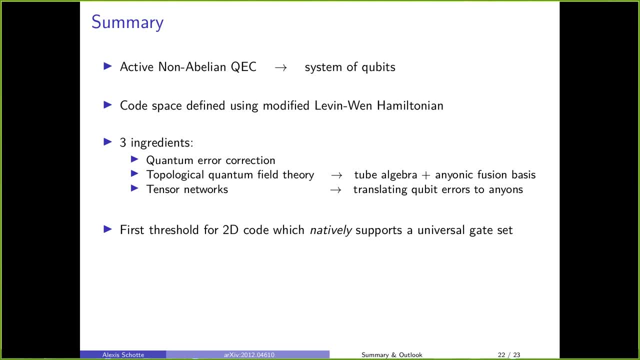 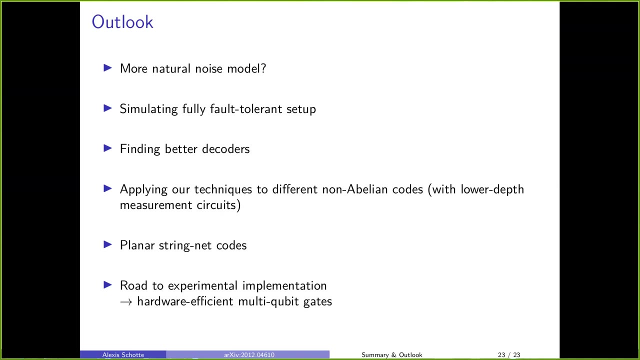 which natively supports a universal set of gates. Furthermore, it's not just a threshold, it's actually pretty high because it's comparable to the surface code thresholds under similar assumptions. So where to go from here? We really hope this opens the door to much more research on non-abelian. 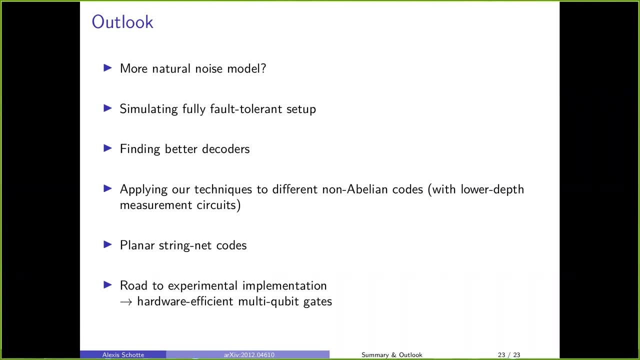 codes. There's many directions to go Just for this project. the obvious next thing to study is generalizing our simulations to a fully fault-tolerant setup. We could also look into better decoders, different noise models. Then there's also other codes that 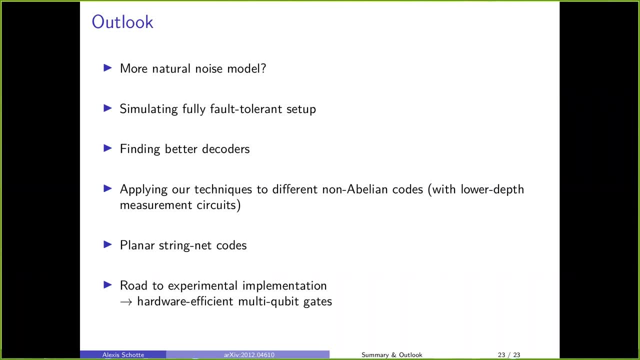 could be studied. We could also look into better decoders, different noise models. Then there's also other codes that could be studied. Our codes have pretty complicated measurement circuits with pretty high depth. There could be other non-abelian codes based on, for example, the quantum double model. 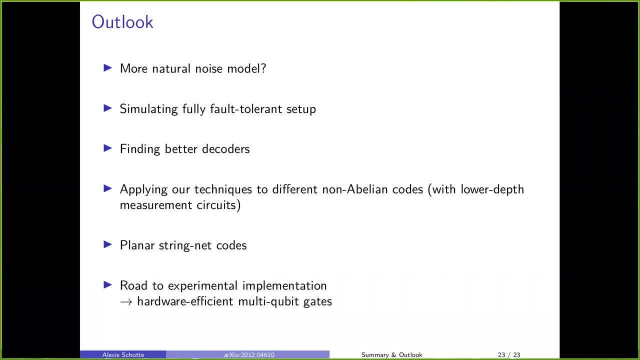 which are simpler, Then you could consider a planar version of this where information would be encoded in. well, you would have punctures containing anions and then your information would be encoded in the degenerate fusion state of these anions. And then, maybe the most exciting one for me, is thinking about some realization of this, So the circuits we need are very high depth. however, if there is a way to do some multi-qubit gates very efficiently on the hardware level, these circuits suddenly are not so big anymore. So this would be the first step, kind of realizing. 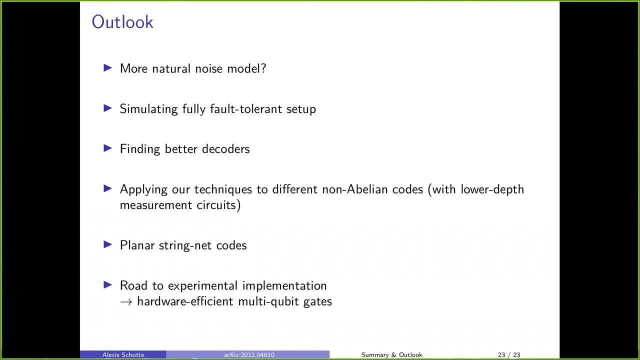 these f moves as an efficient shot in one shot, as an efficient thing would really open the door to to any experimental realizations of these codes. So that's it. That's it for me And I hope I convinced some of you about the importance of studying non-Abelian codes. 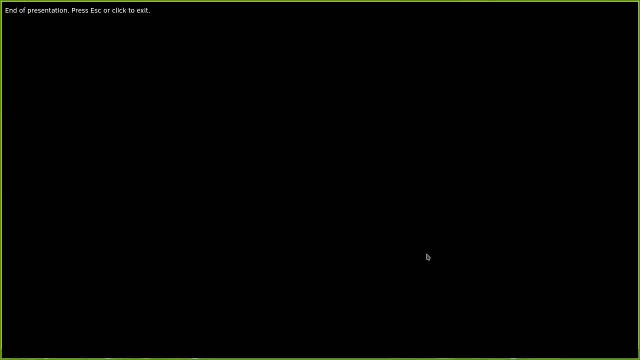 And, yeah, I'm ready to take some questions. Thank you very much, Alexis, for the wonderful talk. There's a bunch of questions going on in the Slack chat, Barbater Hall, And I think some of your co-authors have logged in and are helping answer. 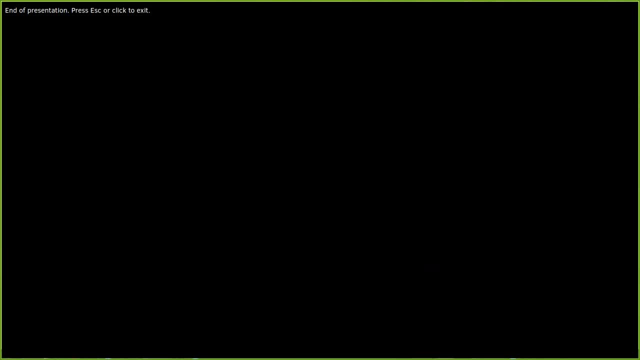 But I'm not sure if I should repeat some of those questions because I believe they've already been answered. But maybe I'll just ask you about something you mentioned in your question session which was in your summary slide. You mentioned planar stringnet codes. 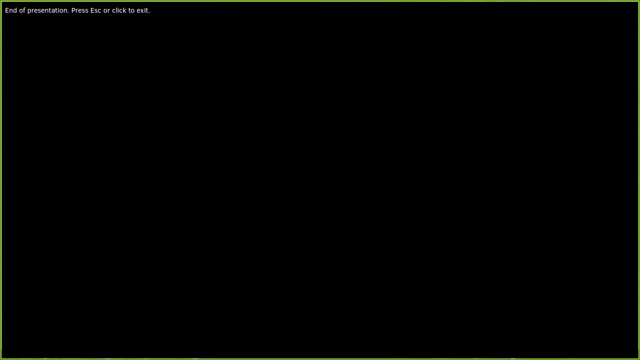 What are the prospects for? I mean, your simulations all involve a Taurus. What can you say about codes that are planar? Well, so we happen to have discussed this before, But you cannot just Like do the same thing as on the surface code. 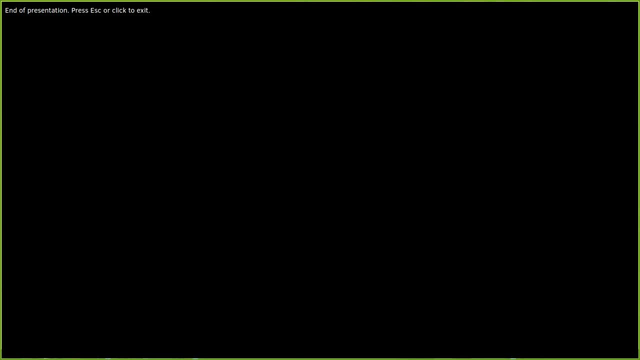 So it really needs to happen with punctures containing anions and then using a degenerate fusion state. So I don't know exactly for the necessary steps to simulate the planar version of this, But it's certainly something we will look into. We haven't really explored that yet. 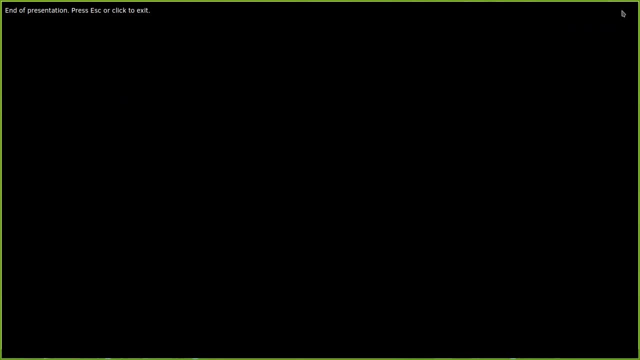 I suppose the first thing you would need would be to choose an encoding. Yes, I see Yeah here on the Taurus version. all you need to do is just check if any errors that happens percolate around you. Non-trivial. 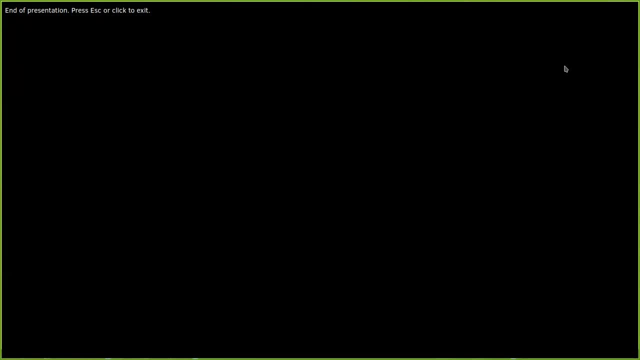 Yeah, Yeah. Well, that's a first order decoder. Of course there are high order things, But presumably these are suppressed And you don't actually need to correct them, right Yeah? So someone, Michael Vassar, asks: is your simulation code? 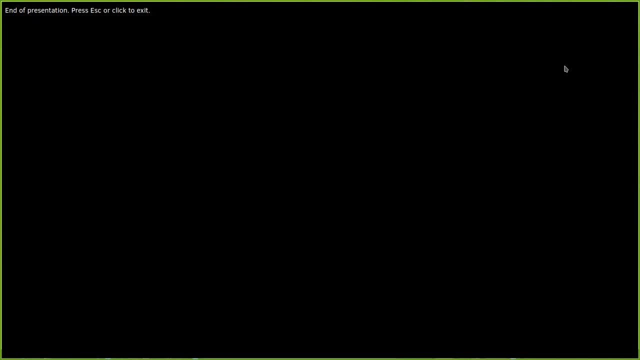 publicly available? Not yet, But it's a very good question. We plan on releasing it to GitHub, But we're still cleaning up the code. since it's a lot of code, We need to add some comments here and there and clean things up. 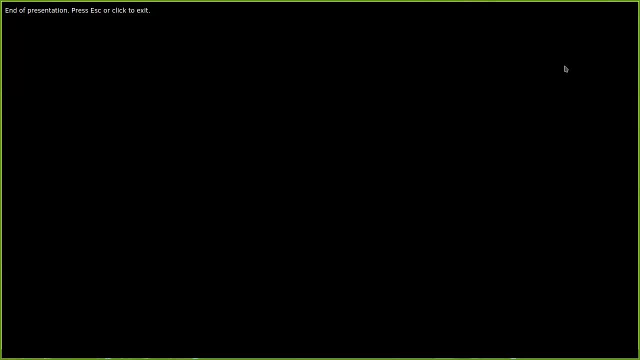 But it will be available on GitHub, All right. Well, we've got you on record saying that now. So the pressure's on, The pressure's on. Yeah, That's good, though It's a lot of work cleaning up code. 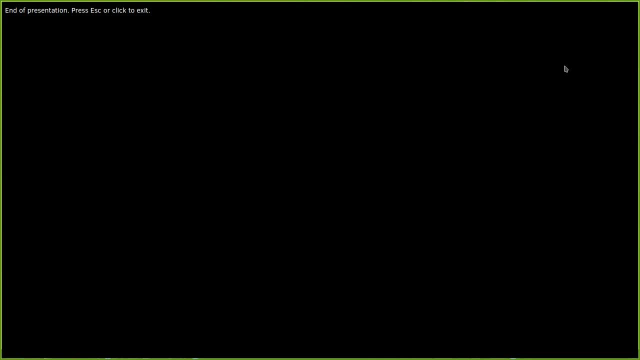 But it's a great resource if you can do it. Someone else, Tom Scrubby, asks. my understanding is that the logical gates in this code or performance are formed via Dane twists. Do you think these operations can be made fault-tolerant? 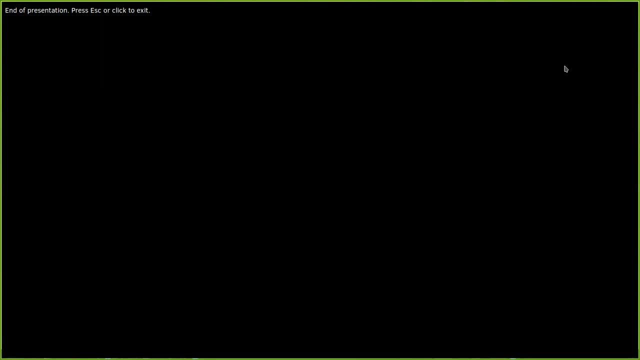 It seems like they will map local errors to non-local ones. To be very honest, I'm not super well-versed in these things. I think there is a way, But I'm sure one of my co-authors would be very eager to talk about this. 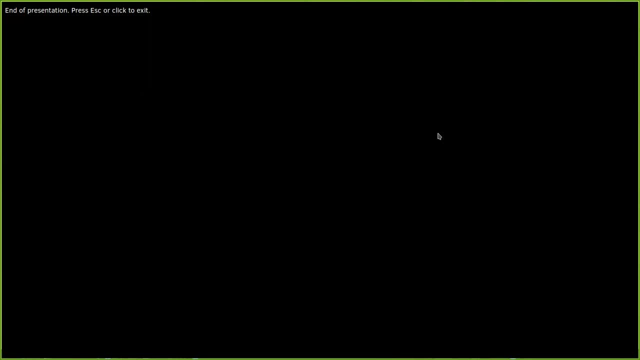 Gwendolyn is an expert on applying Dane twists. Yeah, Dane twists Right. And Barbara Ter-Hall asked about the necessity of applying the unitary operator u sub v. Can you just say a little? I think it was resolved in Slack. 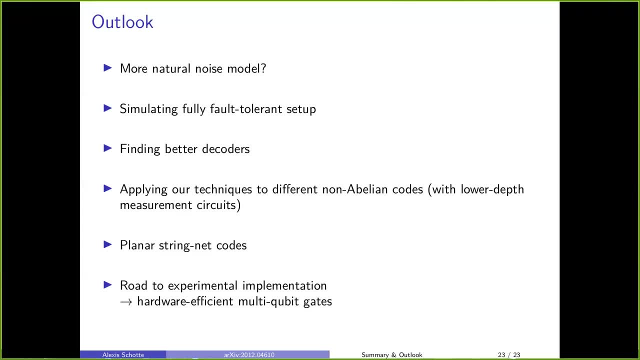 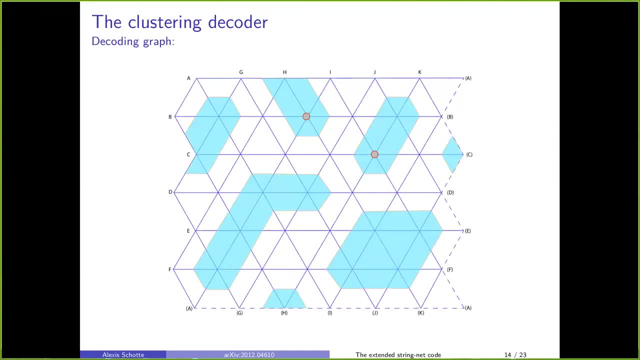 But maybe you could just elaborate. It seems like you really have to actively apply this unitary And then it's not like in stabilizer codes where you can defer a polyframe update until later. Yeah, So let's do it. Maybe comments on the prospects for fault tolerance. 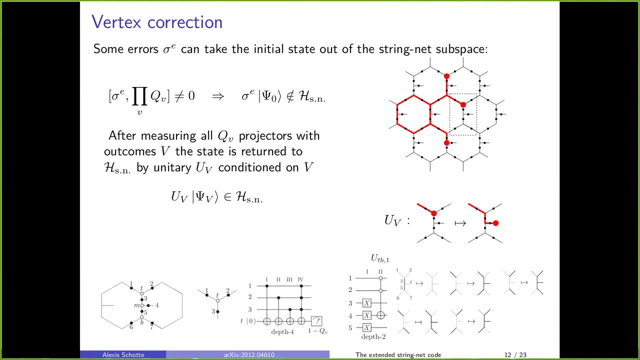 You got about two minutes before we have to start the next talk, OK, So why this is so necessary? Did I understand this well? Why is it necessary? And then, is it necessary? If so, why? And maybe you could comment about the prospects? 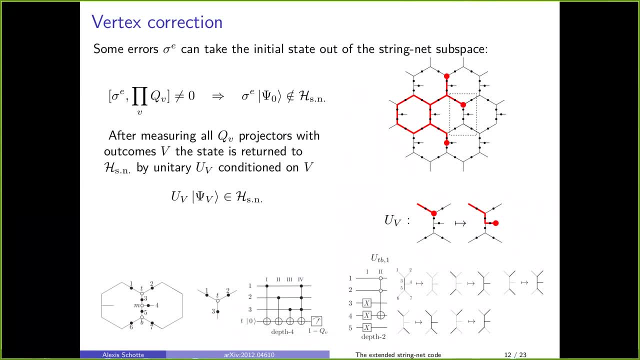 for fault tolerance using these ideas and maybe fault tolerance simulation as well, which I think is linked to the answer to this question. Yeah, So the need for this arises from the fact that, essentially, before correcting, you want to see like you want to see these excitations, that 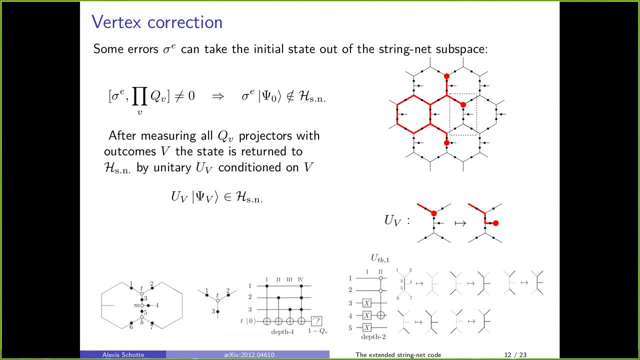 that occur as anions And you can only understand these things as anions. This only makes sense- And it's only well-defined- within this subspace where all your various conditions are satisfied. Once you leave this subspace, it's just a mess of very complicated superposition of states. 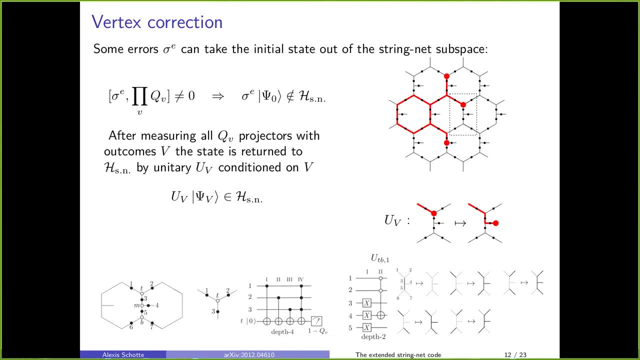 So yeah, So, before you can understand this mess of a state, as- oh, this is just some anions living here And there, you must go back to the subspace. In our simulation we did this like between every error, But in practice you would, just in practice. 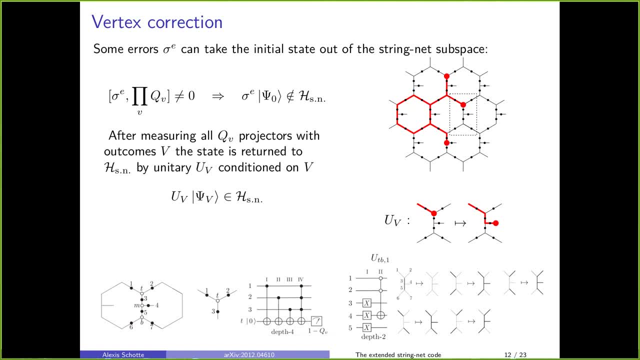 you don't need to do this. You can just noise happens, And then you do all your measurements, You fix your vertices And then you can go on. And we haven't really worked on the prospect of including measurement errors into this thing, since these are necessary before you can measure. actually. 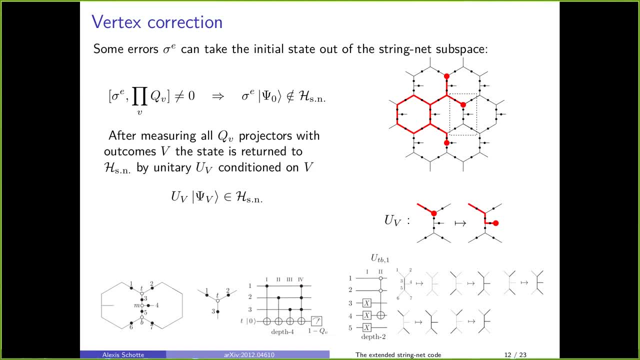 I mean, these things must be applied correctly before you can measure. Yeah, You're any in charge correctly. So we're still working out how that would happen, But I would love to discuss more on this if there is some more time later.